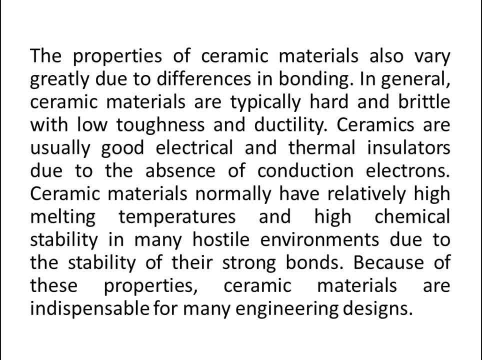 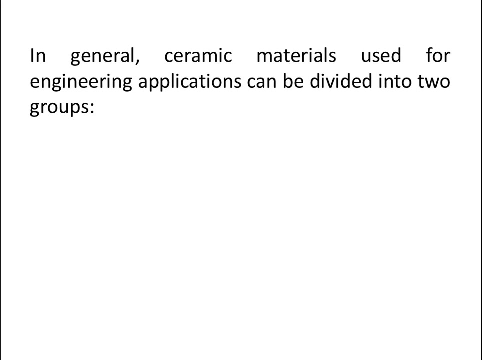 insulators due to the absence of conduction electrons. Ceramic materials normally have relatively high melting temperatures and high chemical stability in many hostile environments due to the stability of the strong bonds. Because of these properties, ceramic materials are indispensable for many engineering designs. In general, ceramic materials used for engineering applications can be divided. 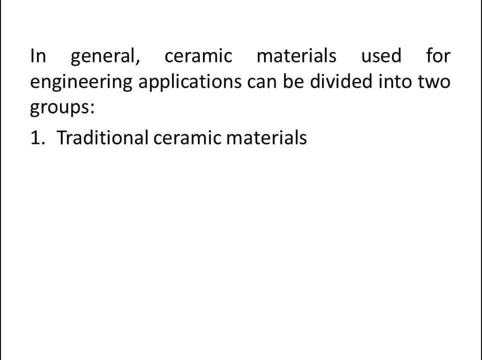 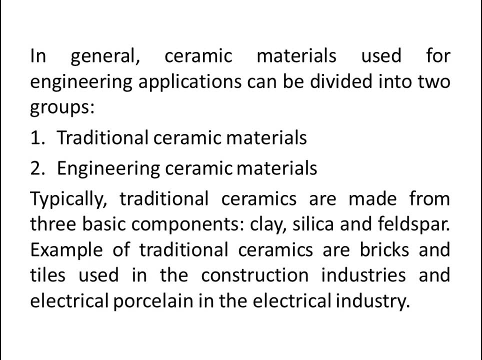 into two groups. First one is traditional ceramic materials and second one is engineering ceramic materials. Typically, traditional ceramics are made from three basic components, and they are clay, silica and feldspar. Example of traditional ceramic is bricks and tiles used in the construction industries, and 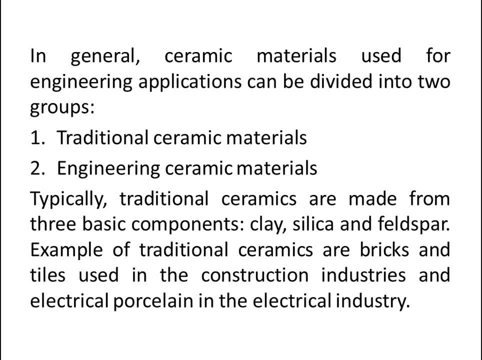 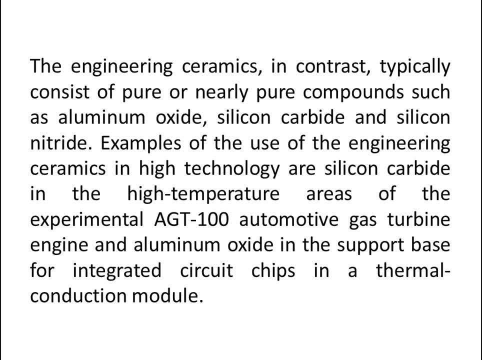 electrical porcelain in the electrical industry. The engineering ceramics, in contrast, typically consists of pure or nearly pure compounds such as aluminum oxide, silicon carbide and silicon nitride. Examples of the use of the engineering ceramics in high technology are silicon carbide in the high temperature areas of the experimental. 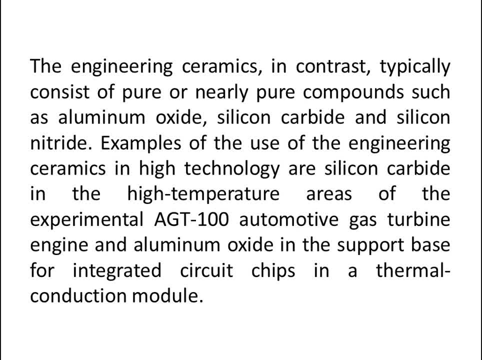 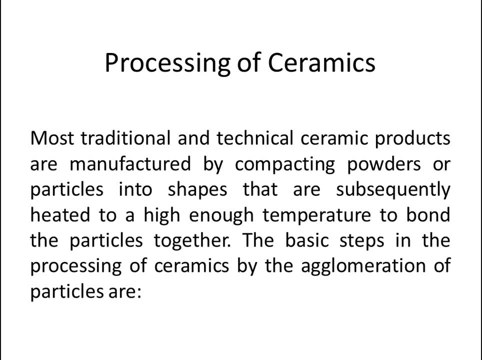 agt 100 automotive gas turbine engine and aluminum oxide in the support base for integrated circuit chips, a thermal conduction module. now let's talk about the processing of ceramics. most traditional and technical ceramic products are manufactured by compacting powders or particles into shapes that are subsequently heated to a high enough temperature to bond the particles together. the 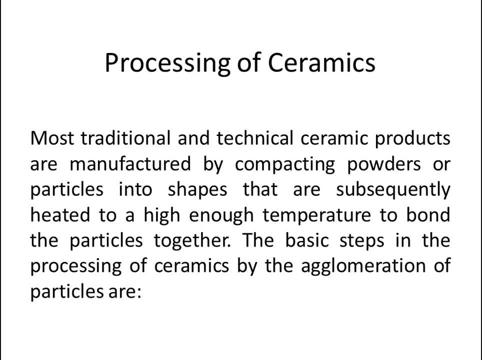 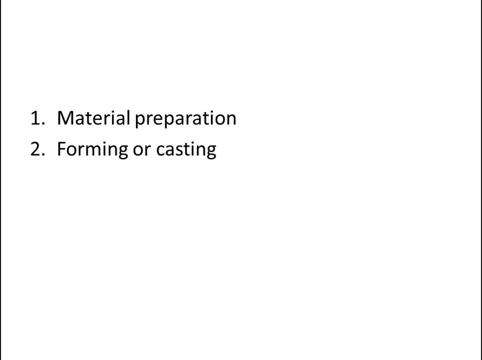 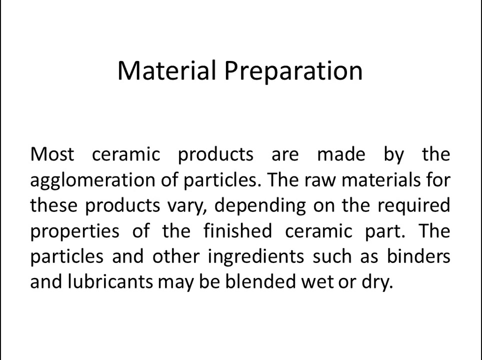 basic steps in the processing of ceramics by the agglomeration of particles are: first, one is material preparation. second one is forming or casting. third one is thermal treatment by drying and firing, by heated the ceramic shape to a high enough temperature to bond the particles together. now let's talk about the material preparation. most ceramic products are made by: 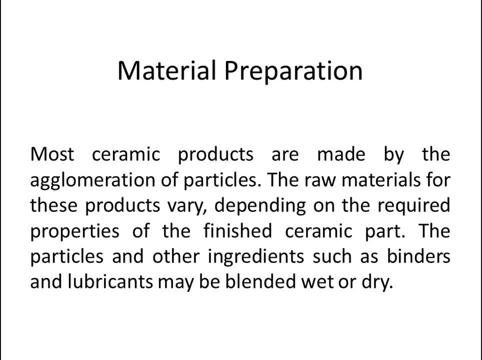 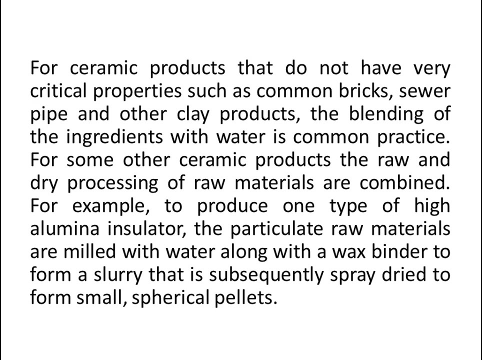 the agglomeration of particles. the raw materials for these products vary depending on the required properties of the finished ceramic part. the particles and other ingredients, such as bindings and lubricants, may be blended wet or dry for ceramic products that do not have very critical properties, such as common bricks, sawyer pipe and other clay products, the blending of the 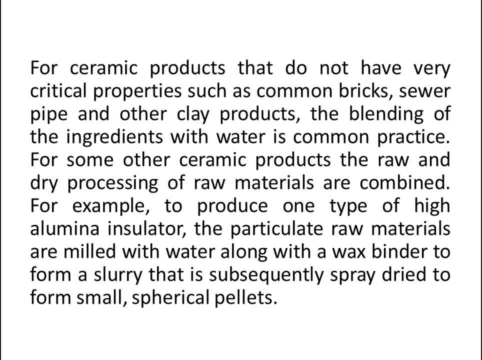 ingredients with water is common practice for some other ceramic products. the raw and dry processing of raw materials are combined, for example, to produce one type of high aluminum material in a insulator. the particulate raw materials are milled with water, along with a wax binder to form a slurry that is subsequently sprayed right to form small spherical pellets. 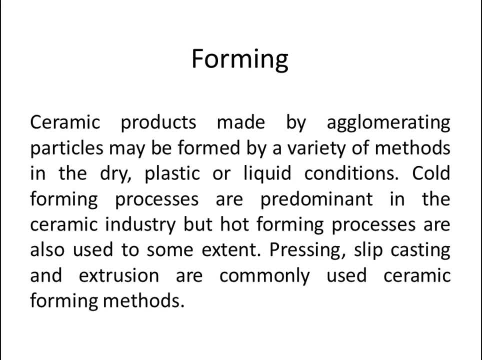 let's talk about forming. ceramic products made by agglomerating particles may be formed by a variety of methods in the dry, plastic or liquid conditions. coal forming processes are predominant in the ceramic industry, but hot forming processes are also used used to some extent. pressing, slip casting and extrusion are commonly used ceramic. 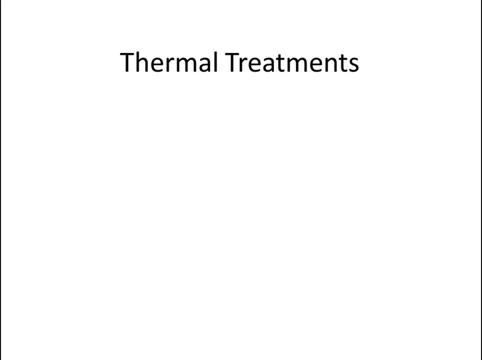 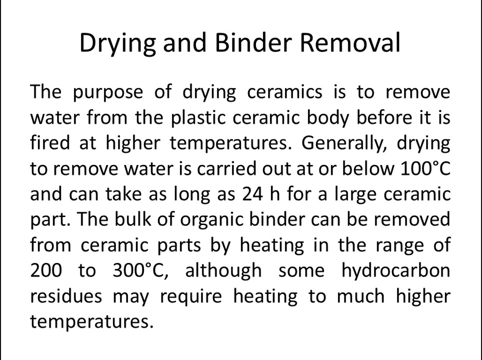 forming methods. now let's talk about thermal treatments. thermal treatment is an essential step in the manufacturing of most ceramic products, and your thermal treatment e-co테 episode. thermal treatments are first one drying, second one is sintering. third one is vitrification and can take as long as 24 hours for a large ceramic part. 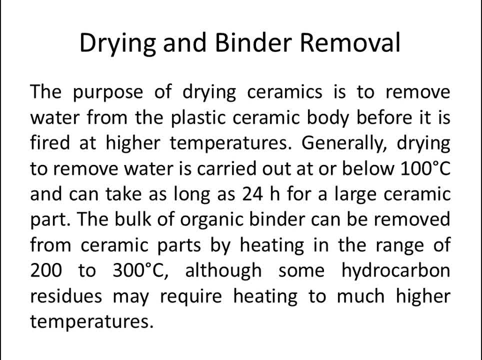 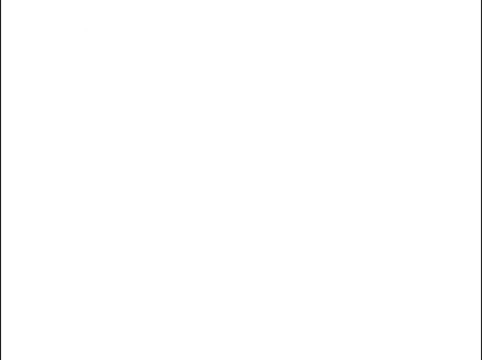 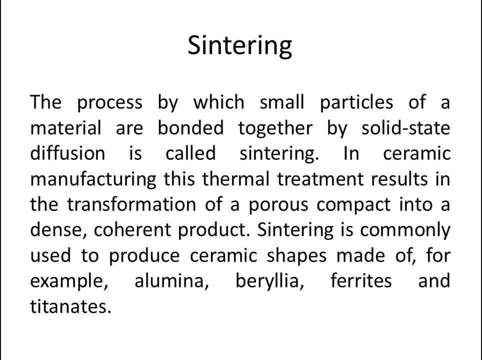 The bulk of organic binder can be removed from ceramic parts by heating in the range of 200 to 300 degrees Celsius, although some hydrocarbon residues may require heating to much higher temperatures. Let's talk about Sintering, The process by which small particles of a material are bonded together.